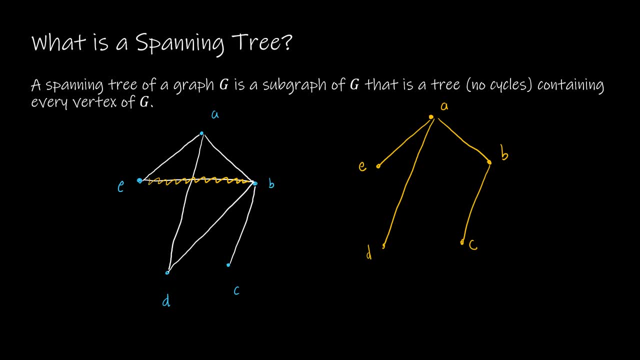 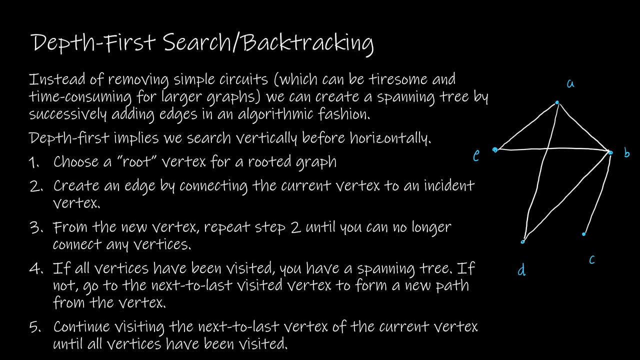 to get to one vertex and simply remove those edges, And so essentially that's what I've done here- is I've created a spanning tree by getting rid of any circuits. So instead of simply identifying where the circuits are and removing any extra edges, we can actually do this by starting with a node and then 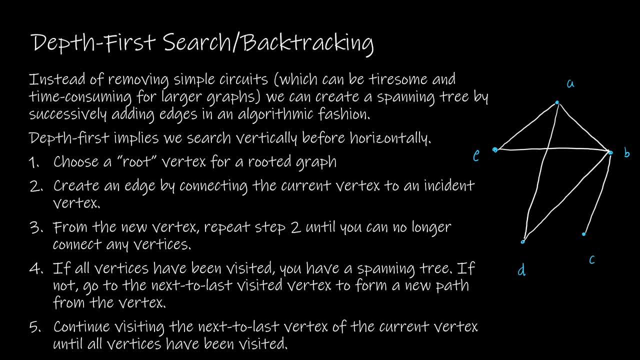 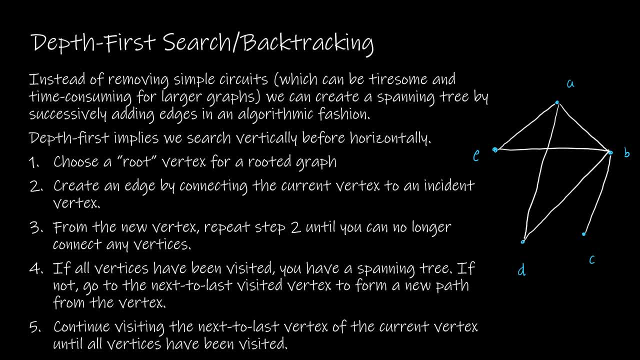 creating new boundaries And with that coming into place, this doesn't have any제this. one will start into something even easier than the original E, which is the personal That's going to be really important. So to, for example, here, essentially what you're going to do when you do including Ordinance is you're 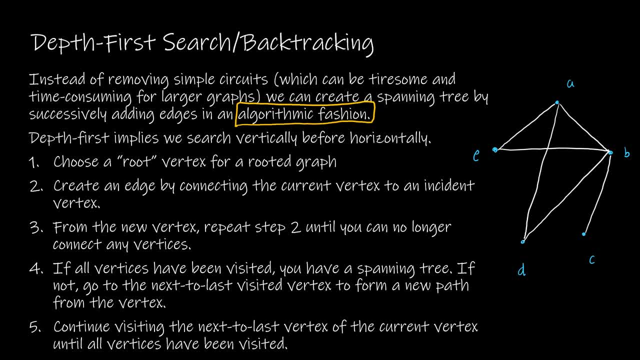 going to do what's called else, the elector sub square, or you're going to do what's called 49. This king of decentralized proof It is. you're going to call Dolin masters, heads of computers, computers, computers. Of course you're not going to take a new findet. Alright, A $60 is going to. 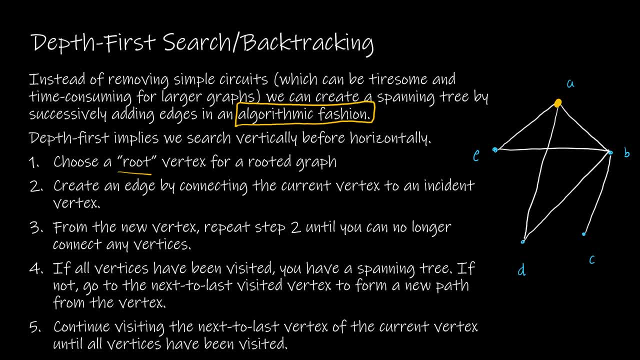 The next step says: create an edge by connecting the current vertex to an incident vertex. So it really doesn't matter if you have edges that are labeled in an ordered fashion. So, for instance, we have the alphabet, And so if we wanted to connect these in alphabetical order, obviously I would choose B over E. 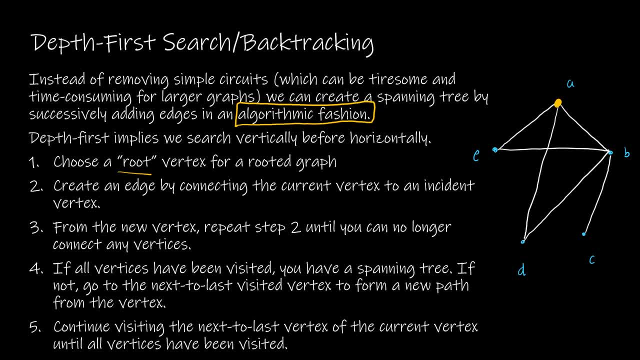 So I would examine from A that I could connect either E or D or B, because those are all the vertices that are connected to A and I can choose any one that I want. So for instance, let's say I choose B, So I'm going to choose B and connect that edge. 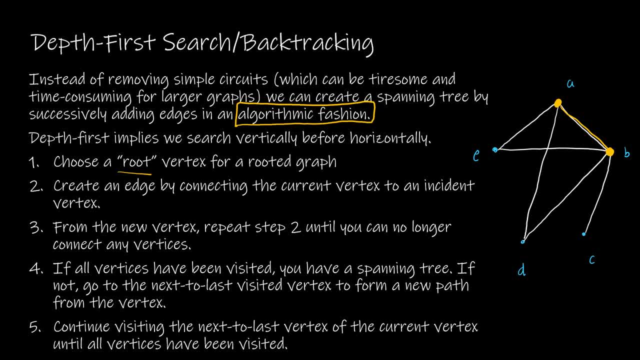 Now the trick here for the depth- I'm sorry, the depth first search is that I don't go back to A. I start at B and say: where can I go from B? Well, B, B would take me to C. So then I look at C and say: well, C is not connected to anything. 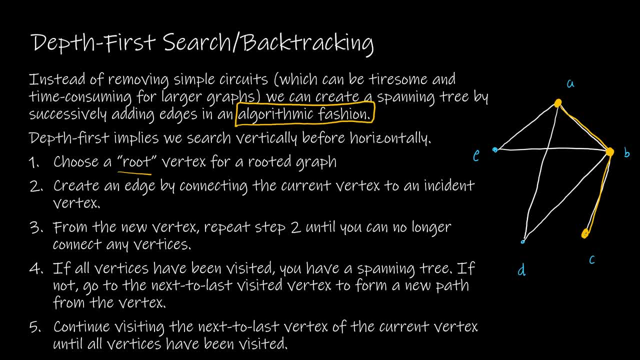 else. So then the algorithm says: if you've gone as far as you can and you still haven't visited all the vertices, go back to the previous vertex. So I'm going to go back from C to B. So that's why it's backtracking. 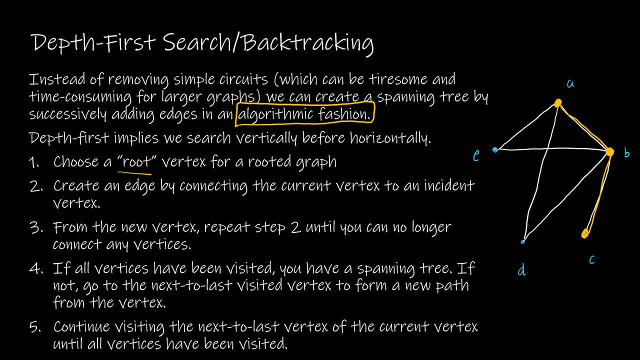 So I'm back to B, And now I'm going to connect anything from B. So I'm going to connect B to D, Okay, And then D connects to A, but I've already visited A, So I can't connect anything to. 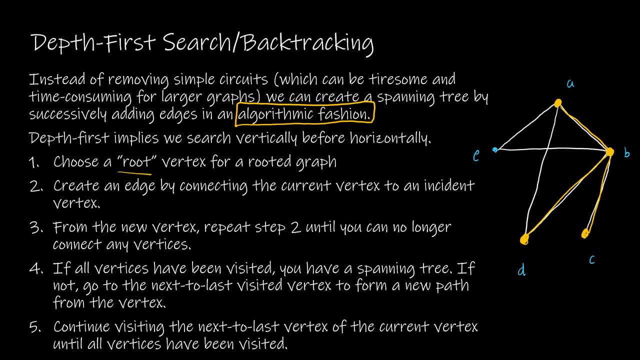 D. So I would go back to B again and say: well, that connects to E. So one example of a spanning tree is starting at A, going to B and, if you'll notice, B branches off into C and D and E. 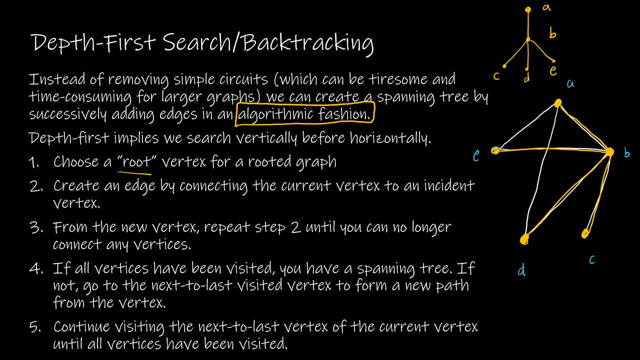 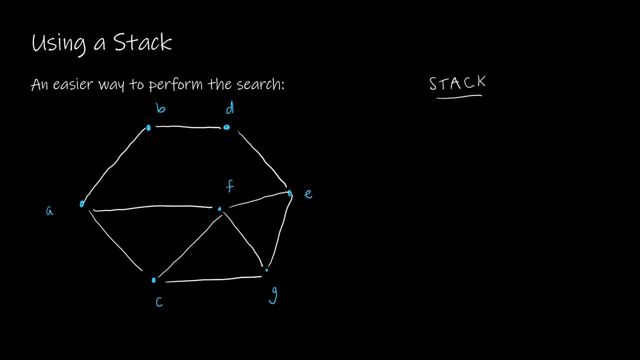 So this is one example of a spanning tree that was created using our depth-first search algorithm. What you'll see quite often- and this is not the way that it's shown in your textbook, but quite often you'll see using a stack to keep yourself organized. 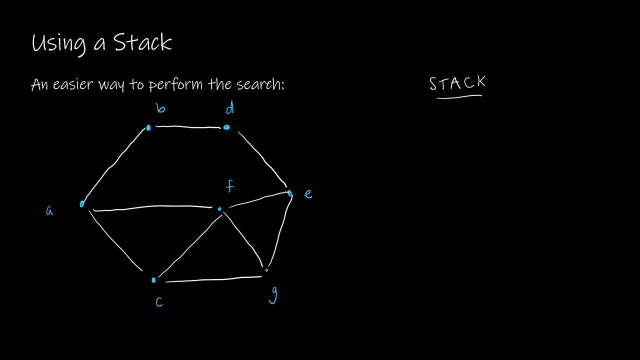 And so here's how that would work. We would start with our root node, So we're going to start with A And I'm going to go back to B, Okay, Okay, So I'm going to go ahead and put visited over here. 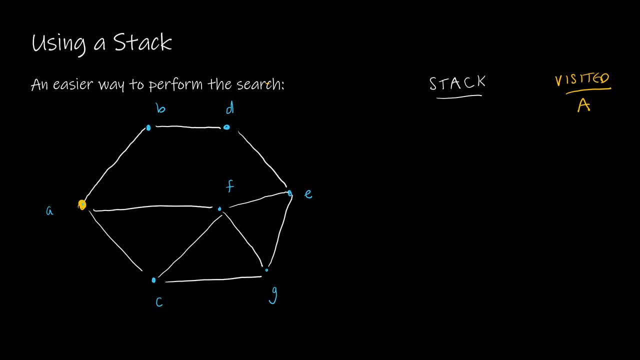 So if I start with A, I have visited A And in our stack we're going to add any vertices that are next to or adjacent to A. So in this case that would be B and C, And we can choose either B or C. So let's say I choose B. So now B is going to leave the stack and I will. 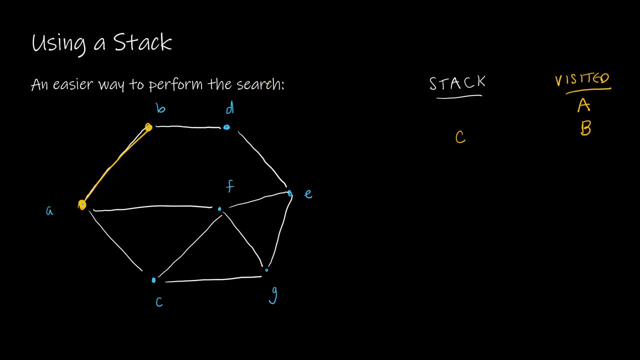 say that I have visited B. Now C is still in the stack, meaning it's still something I can get to. But remember, our algorithm says: now you're going to go from B, So instead of leaving C at the top of the stack, C is going to move down. 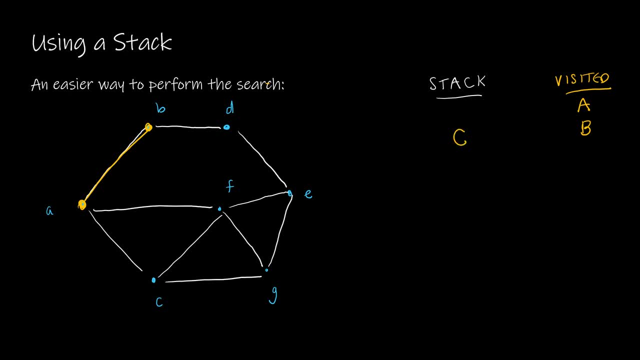 Oops, And we're going to put any vertices adjacent to B, which would be D, And so then I'm going to visit D, Okay, Great, Okay, Okay, write anything adjacent to D. so I'm going to replace D with E, so now E is. 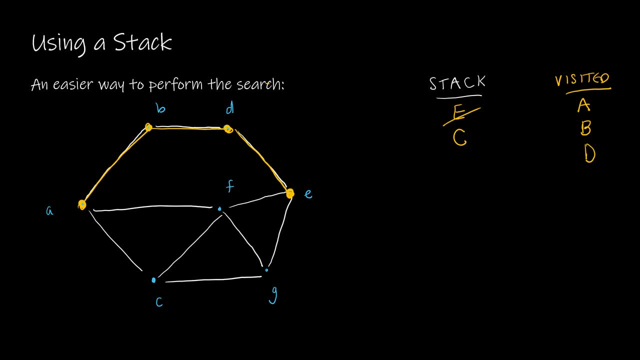 visited, and then from E I can get to either F or G. well, C is still in our stack, but it keeps getting moved to the bottom again because, because it is adjacent to A, so we're going to keep C in the stack, but again we're going to 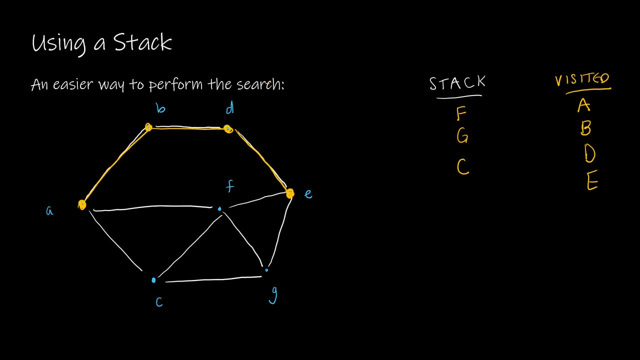 keep going from E. we're going to go as far as we can with E, so I'm going to visit F and then I'm going to write anything adjacent to F, so I'm going to have G or C. so now, notice, G and C were already in our stack, so now I'm going to 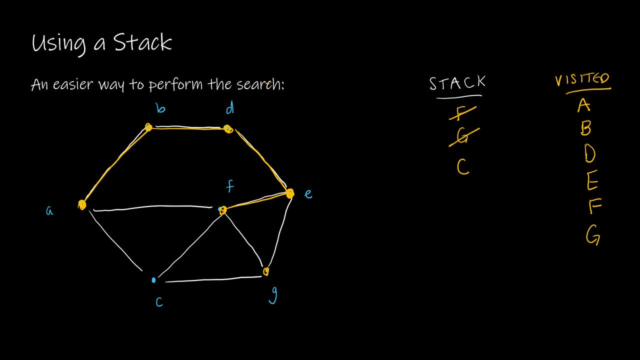 visit G, again from F and then from G over to C. so now I have visited all of the vertices. what does my spanning tree look like? well, it's just a path: A, B, D, E, F, G, C. so that is what my spanning tree would look like in this case: starting from A and making the decisions that I 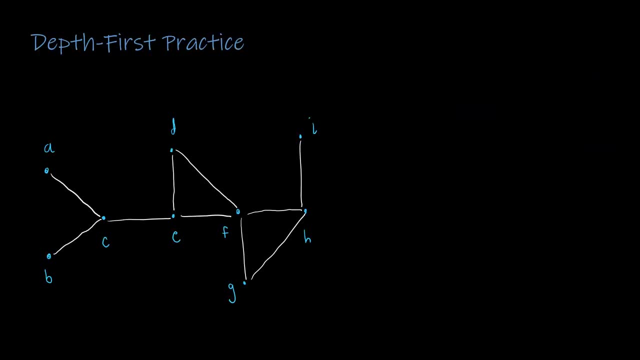 did. here's a practice for you to try on your own. so go ahead and press pause, try this question and then press play to see how you did again. it's important to remember that there's no right answer. there's no one right answer. as long as you're able to visit each of the vertices you have a spanning. 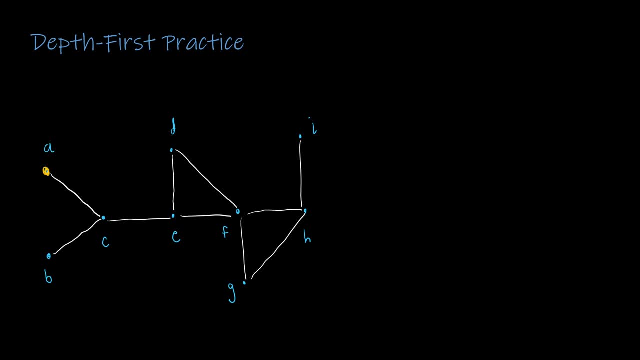 tree. so I'm going to start at A and instead of creating a stack, this time I'm just going to circle potential vertices as we go. so from A, the only potential vertices C, and so we're going to visit C. from there, I can visit either B or E, and just for fun, this time I'm going to visit B. so now E has been. 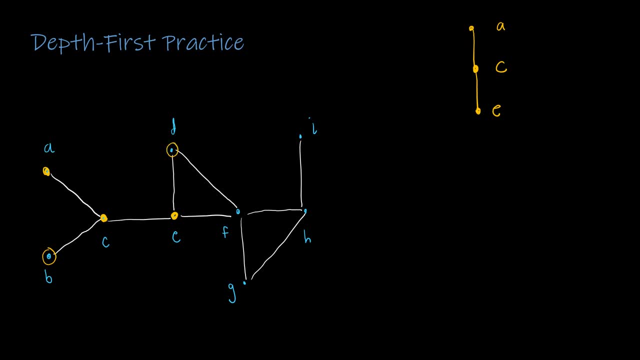 visited. B is still in the stack. from E, I can visit D or F. I'm going to choose D, and from D I can only choose F. so F again leaves the stack and is now visited. from F, I can visit G or H. I'm going to choose G, oops, and then from G, I can. 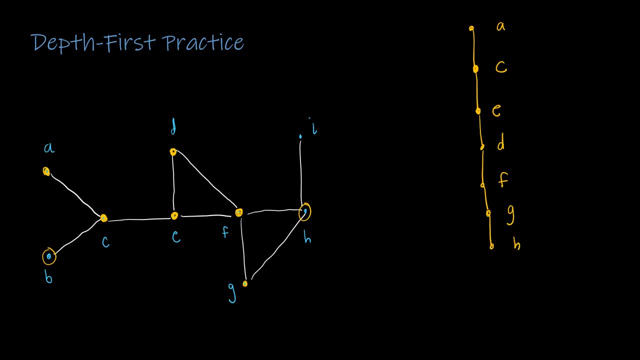 only choose H. so now I have visited H and then from H, I can only visit. oops, I should have been creating the actual tree as I go. from H, I can only visit I, and now I have to backtrack all the way back to C to get this very. 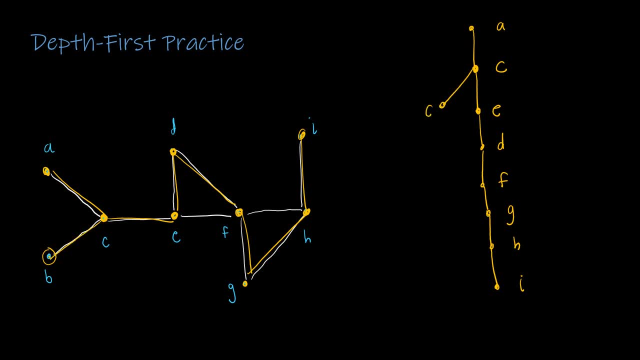 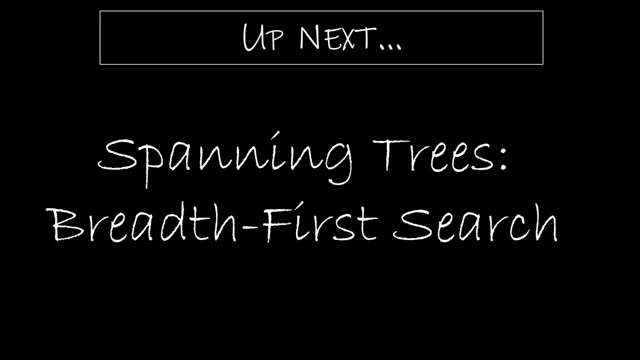 last vertex of B, oops B. so this is one possible spanning tree that you could have come up with, creating our depth first search. next we're going to take a look at another method for creating a spanning tree using a breadth first search. 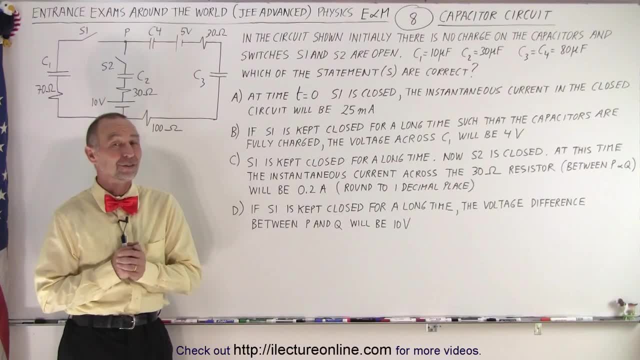 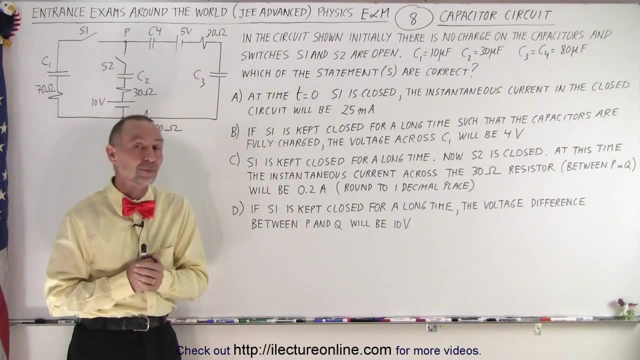 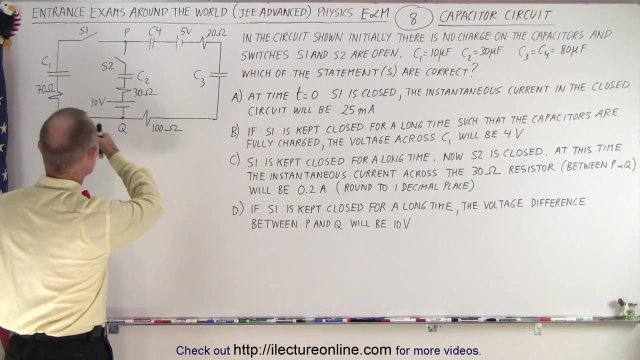 Welcome to iLectra Online. Now here is a definitely a challenging problem out of the JE Advanced Test. It deals with electricity, magnetism, but more specifically with capacitor circuits. And it's not a simple circuit. It has two switches, one, two, three, four capacitors. 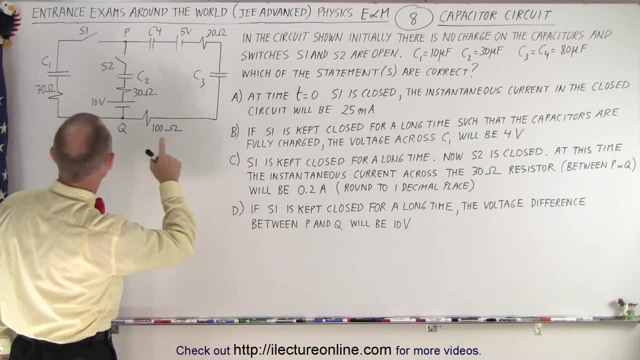 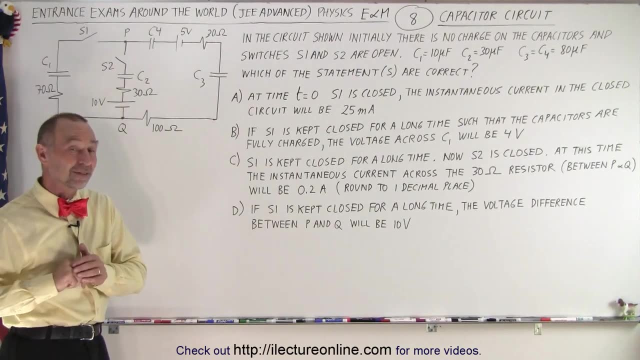 two batteries, one, two, three, four resistors and the switches are closed at different times. Wow, Well, let's read the problem and see what we're going to do with it. It says that in the circuit shown initially, there's no charge on the capacitors and both switches- S1 and S2, are open. 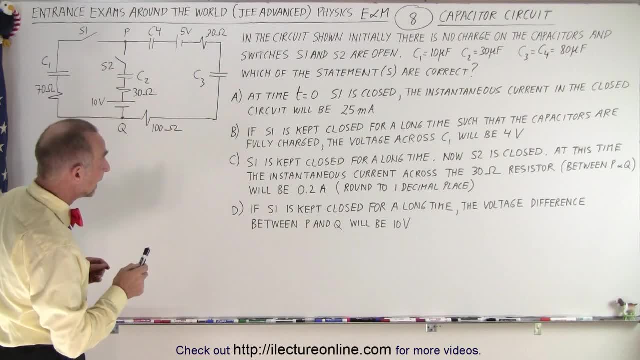 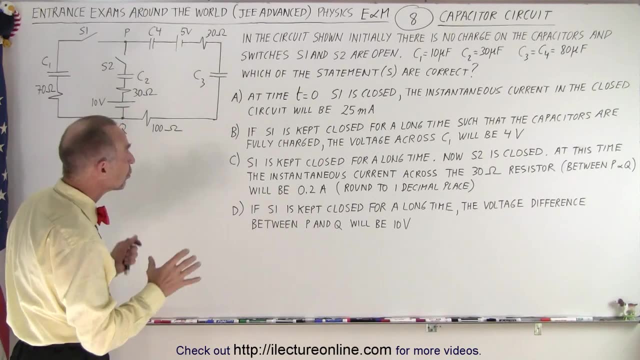 They give us the values of the capacitors- There's four of them- And then they ask us which of these four statements are correct. What I always would prefer that you do- I would recommend that you do that- is put in the capacitor values on the circuit, Because if they're like that on the side,